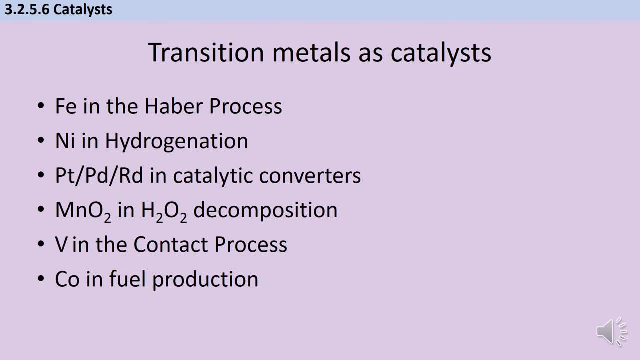 tend to use catalysts like platinum and palladium and rhodium. When you first learned about catalysts, chances are you did an experiment where you looked at the decomposition of hydrogen peroxide with lots of different catalysts and the best one that students are usually allowed to use. 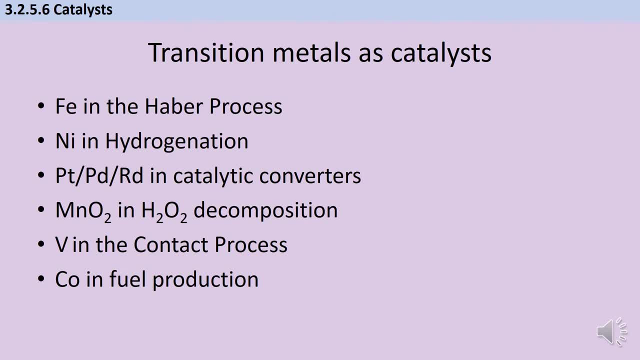 is manganese dioxide, And then more recently, you may have also heard about vanadium being used in the contact process and also cobalt being used in fuel production. As you know, the hydrogen peroxide is used to make hydrogen peroxide and the manganese peroxide is used to make hydrogen peroxide. 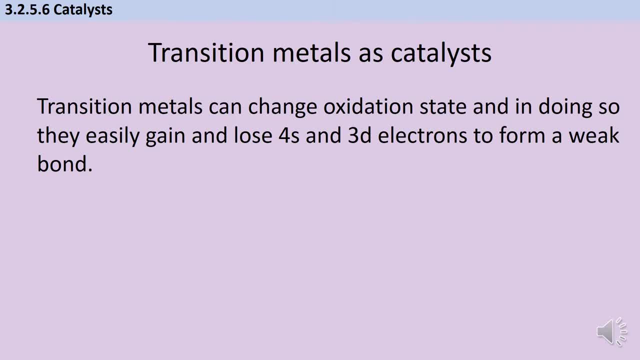 Transition metals have multiple stable oxidation states, and this is linked to what makes them such good catalysts. As they're moving between those oxidation states, they obviously need to be able to readily lose and gain their S and D electrons, and the fact that they're able to do that allows 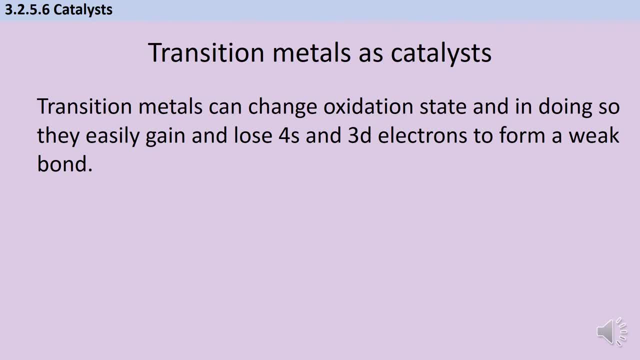 them to make really quite weak bonds with the reactants they're trying to catalyse. This means that transition metals tend to make good catalysts, whereas metals from, say, group 1 or group 2 are far less likely to be good catalysts. So if I was asked to explain why it is that, 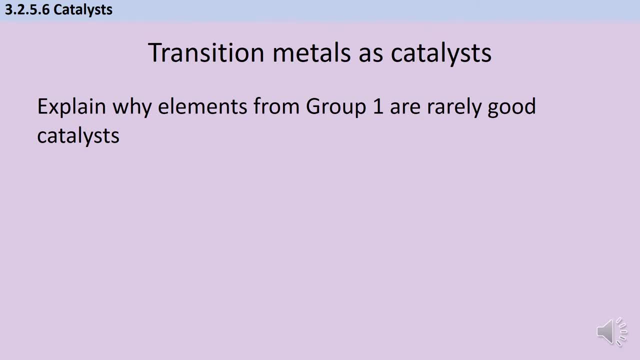 transition group 1 are rarely good catalysts. I want to bring this back to electron configuration. and what is it that is special about the transition metals? So I'd be saying they don't have incompletely filled D subshells and because of that they only exist in a single oxidation. 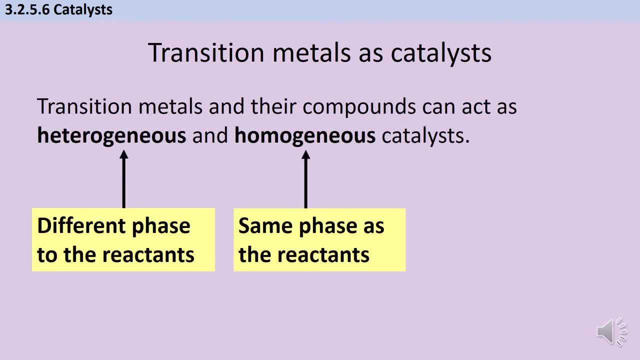 state. We can put catalysts into different groups based on whether they're in the same or different phase to the reactants that they're catalyzing. For the purposes of A-level, you can think of phase as being exactly the same thing as state. So say, if I have a solid catalyst, 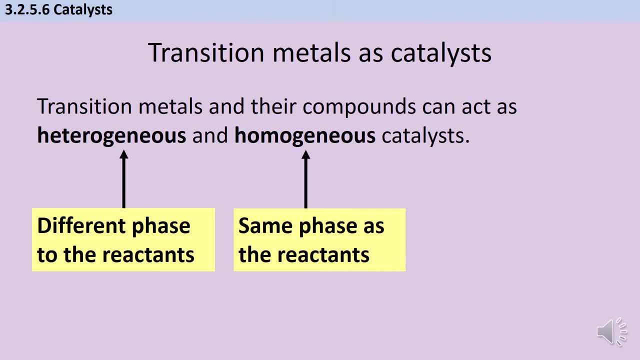 which is catalyzing the reaction of two gaseous reactants, then that would be an example of a heterogeneous catalyst, because it's in a different phase to the reactants. On the other hand, if I've got a catalyst that's in solution and it's catalyzing reactants that are also aqueous and 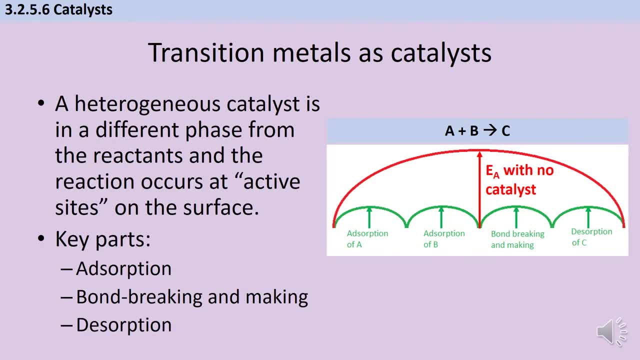 also dissolved, then that would be an example of a homogeneous catalyst. Heterogeneous and homogeneous catalysts work in different ways. As we've just said, a heterogeneous catalyst is one that's in a different phase from the reactants, so that's usually going to mean a solid catalyst. 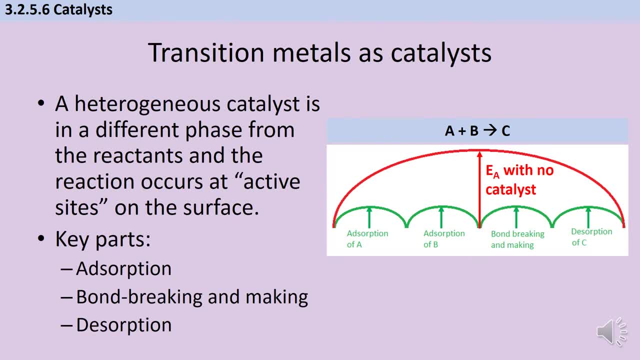 catalyzing the reaction between liquids or bonds, And on the surface of that solid catalyst there are active sites. Active site is a term you've almost certainly heard applied to biological catalysts like enzymes when you did GCSE biology. but you may not have realized that chemical catalysts also have active sites And that's. 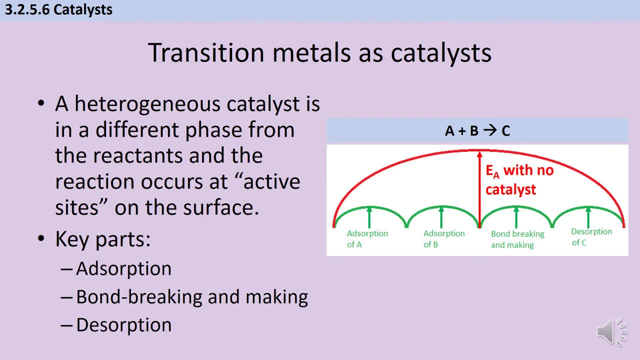 the name we give to the region where the reactants are going to adhere and interact with each other, And it's going to be particularly important when we start thinking about chemical catalysts being poisoned and how they can stop working. There are three key stages of chemical catalysts. 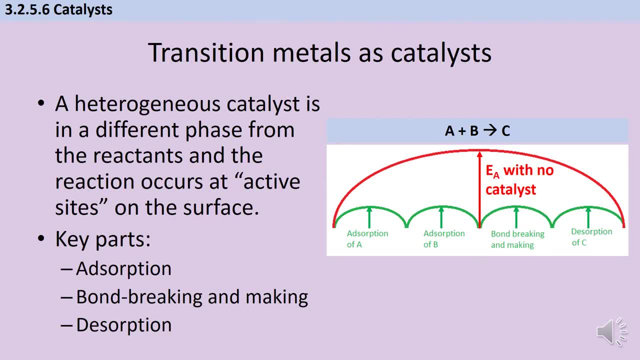 There are three key stages to the working of a heterogeneous catalyst. The first one is adsorption, and that's not spelling mistake. It really is adsorption with a D rather than a B, So, whereas absorption means that something's being taken inside, 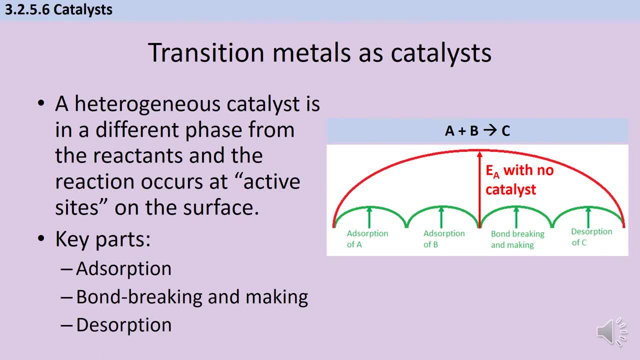 adsorption means it's sticking to the outside. So what's going to happen is that the reactants are going to literally adhere to the active site And for a transition metal, that's going to happen when the transition metal changes oxidation state by either reduction or oxidation, So electron. 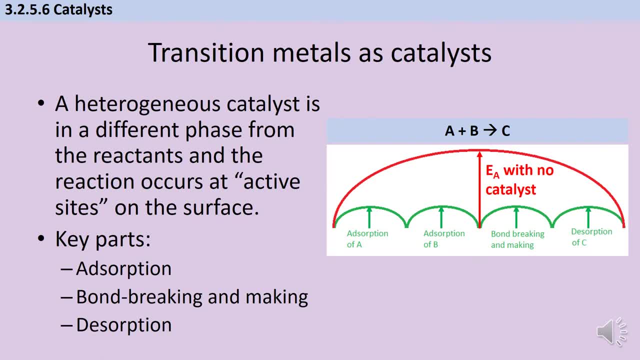 metal and the reactant, And when that happens it's either going to be oriented in a way that makes it easier for it to interact with the other reactant or it might just mean that energetically it's in a more favourable conformation to have bonds broken. So in the second stage is the bond. 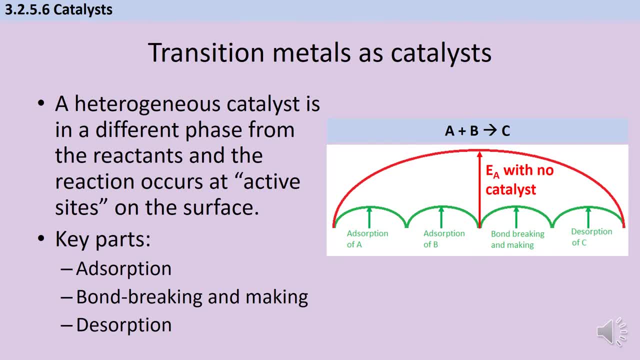 breaking and the bond making, and then the final stage is desorption, And desorption is the opposite of adsorption, so the newly made products are going to be released. When all this is happening. the strength of the bonds between the reactant and the transition metal is crucial to whether 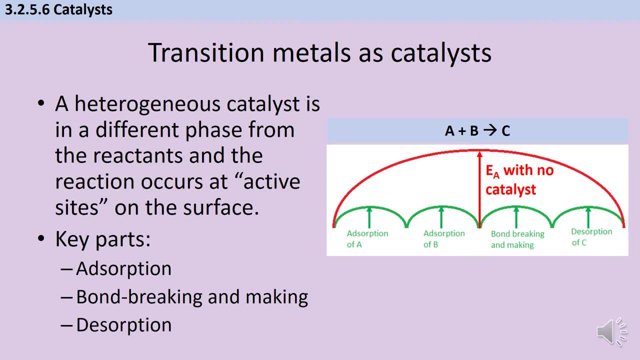 or not a particular transition metal is an appropriate catalyst for a particular reaction. If the interaction is too weak, then the reactants might move away before they've interacted with each other, before they've been brought together, and so no catalysis would happen because no reaction. 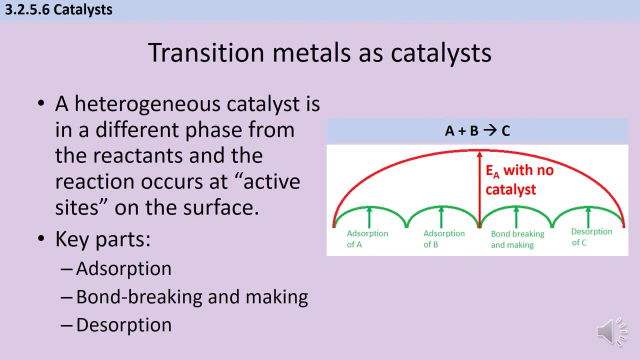 would happen, And this sometimes happens- with metals like silver, so silver doesn't tend to be a very good transition metal catalyst. On the other hand, if the interaction between the reactants and the transition metal particles is too weak, then the reactants might move away before they've been. 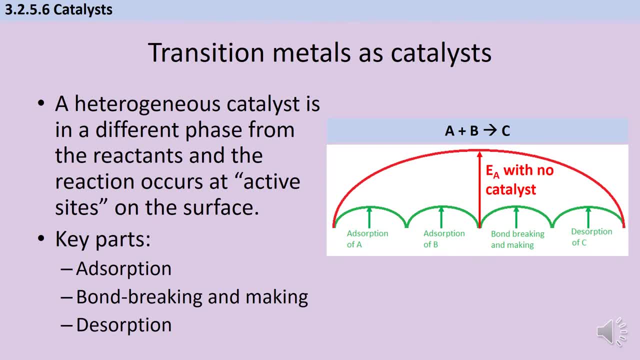 brought together. If the interaction between the reactants and the transition metal particles is too strong, then even though the reactants would be brought together, they would never desorb, And so the active site of that catalyst would just be blocked, because it would still have. 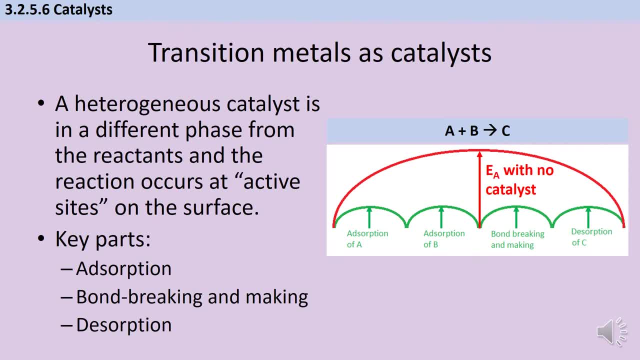 the original atoms in it. So for instance, tungsten tends to have this problem. It can catalyse the reaction, but then the products never desorb, so it can't ever be used again. So that's not a great catalyst either. You might wonder how, having all these extra stages, 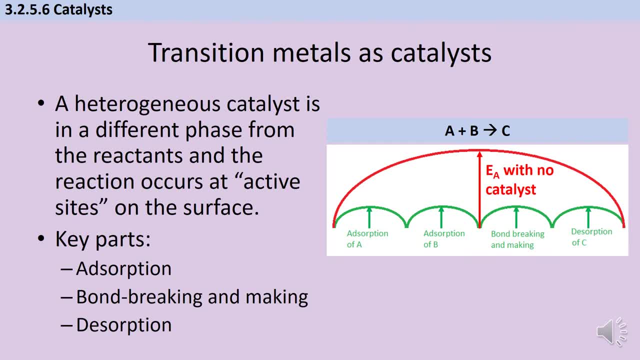 helps the transition metal to be a catalyst. Well, each stage has an activation energy, But because these are happening independently of each other, those activation energies are separate. You don't need to have all of the energy for the whole reaction in one go. You can have just enough energy to make something. 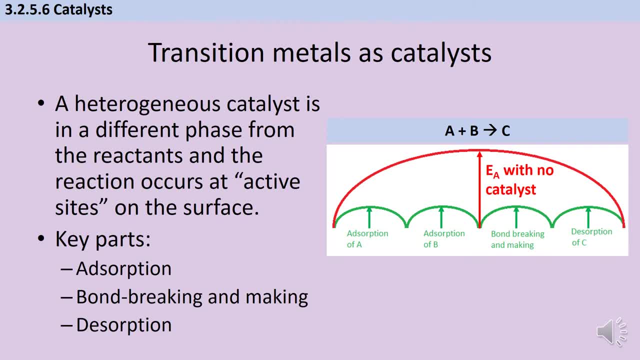 adsorb and then you can have just enough energy to break the bonds and so on. So if you look at this diagram over here on the right, we've got an example of a reaction where A and B react to form C. So there's a small activation energy for the adsorption of A. 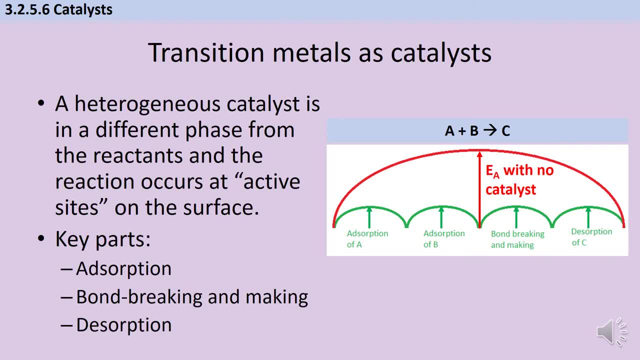 and a small one for adsorption of B, And then there's the activation energy for breaking the bonds And finally there's the energy required to make the product C desorb. But they're all quite small activation energies And while if we added them all up together we might need as much energy as the whole reaction. 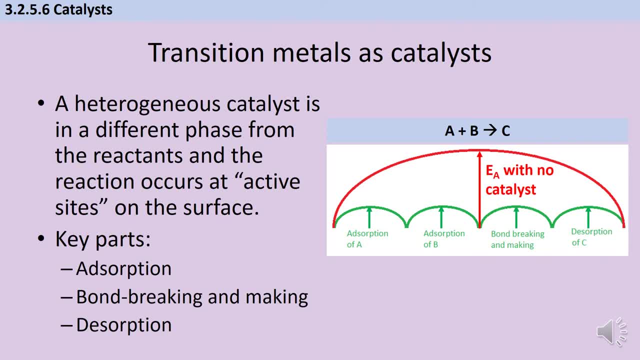 because the reaction has been broken down into these intermediate stages. you don't need all the energy in one go, So if a particle has a bit less energy, it can still proceed through the reaction, provided it's interacting with the catalyst. Many of these transition metal catalysts are really quite expensive. 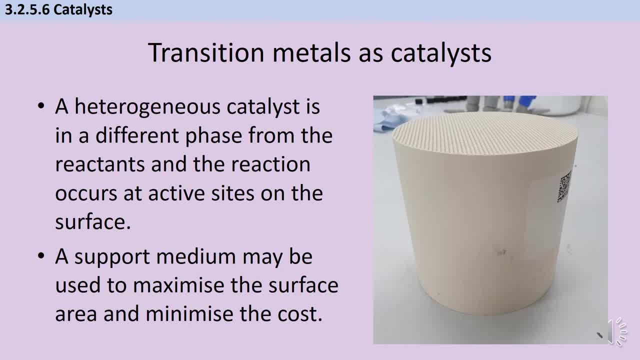 So one of the aims of industry is to use as little metal as possible to catalyse the reaction, And so, in order to do this, they want to maximise the surface area of that catalyst so that if you have, say, a gram of platinum, 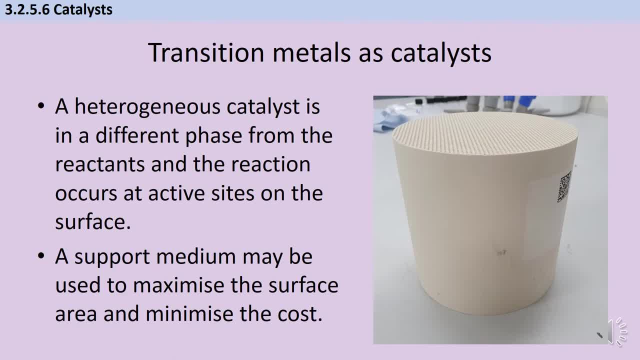 it can catalyse as many different reactions as possible, And one way to do this is to use some kind of support medium to maximise the surface area. So cars have catalytic converters in them and they have either a platinum or a palladium or a rhodium catalyst. 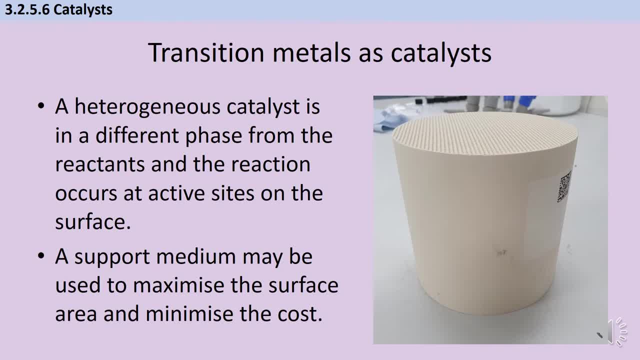 And so the precious metal, rather than just being left in a lye, is mixed into a paste, and the paste is spread over a ceramic support like this one here, And that's going to allow the platinum or palladium or rhodium to have the biggest possible surface area, because it's really spread out. 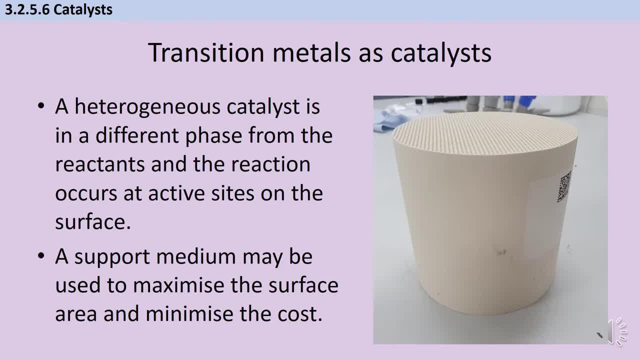 And as the exhaust gases filter through this kind of honeycomb structure, it's going to have the maximum number of opportunities to interact with that catalyst And that's going to sort of make the whole thing just work really well and therefore minimise the cost, because you're not having to pay for extra catalyst to go into the car. 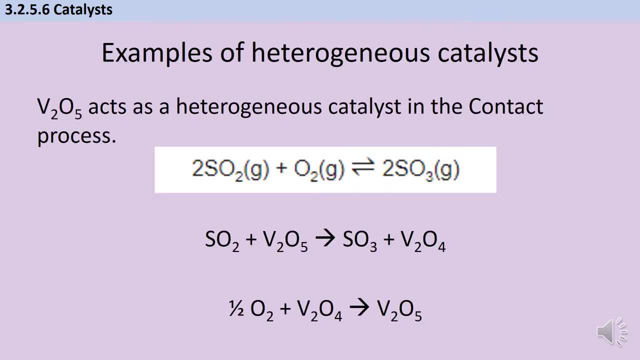 The contact process is the name given to a series of chemical reactions which are used to produce large quantities of sulphuric acid in industry, And it's also named in the AQA specification as an example of a chemical reaction that has a heterogeneous catalyst. 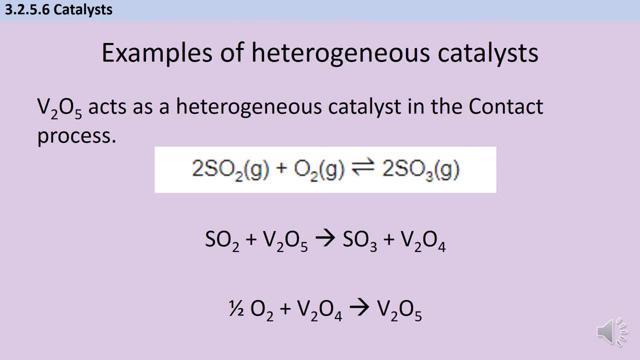 One of the first stages of the contact process is the reaction of sulphur dioxide, which is a gas with more oxygen, which is also a gas to make sulphur trioxide, which is also a gas, And this can be catalyzed really well by platinum, which is also a transition metal. 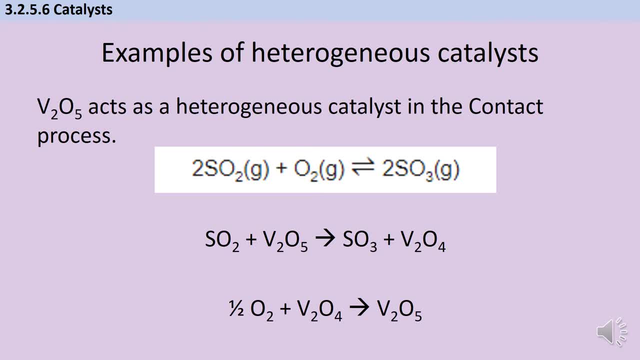 But one of the problems with platinum- apart from the fact that it's really expensive and quite rare, is that it's easy for it to become poisoned by arsenic. So what that means is that the arsenic will adsorb to the active sites of the platinum and then doesn't desorb. 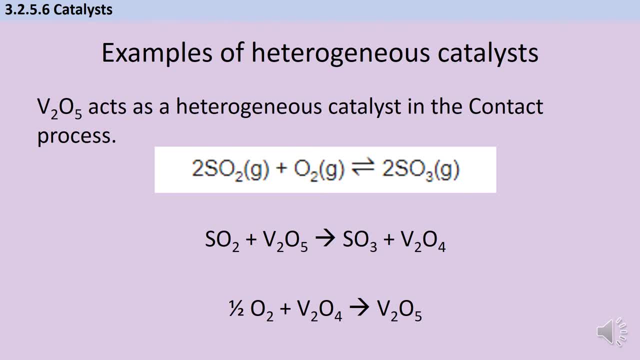 And unfortunately, the sulphur feedstocks that are used to produce the sulphur dioxide quite often have arsenic impurities, So nowadays we tend to use vanadium pentoxide as a heterogeneous catalyst instead. Now, in describing this chemical reaction, you need to know these two equations. 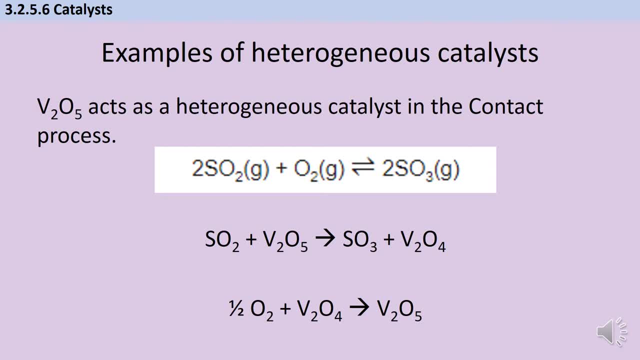 and you need to be able to show how the change in oxidation state of vanadium allows it to act as a catalyst. So here in the vanadium pentoxide, we know that the oxidation state of oxygen is always going to be minus two. 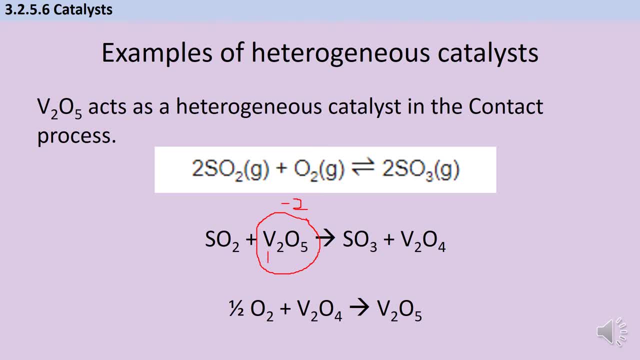 And there's five of them and there's only two vanadiums, So that is going to have an oxidation state of plus five. So then, when that reacts with sulphur dioxide, sulphur trioxide is produced and the vanadium is reduced from an oxidation state of plus five. 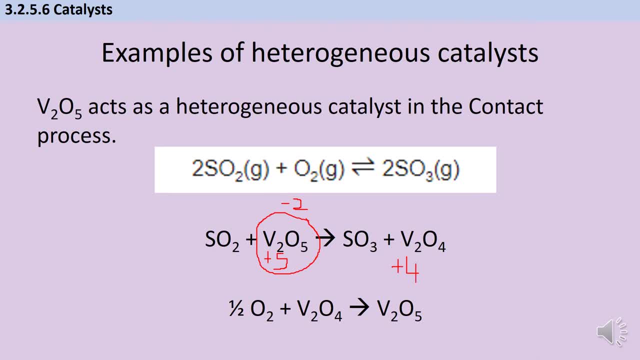 Down to an oxidation state of plus four. So that's my first reaction. And then, because vanadium is acting as a catalyst, or vanadium pentoxide is acting as a catalyst. you know that a catalyst can't be used up and it can't be changed by the chemical reaction. 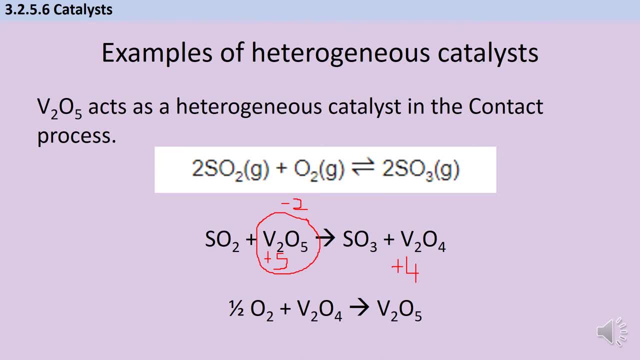 We have to get it back in the form that it started in, So that vanadium oxide is then going to react with half a mole of oxygen to return it back to this plus five oxidation state instead. So you need to know those two chemical reactions. 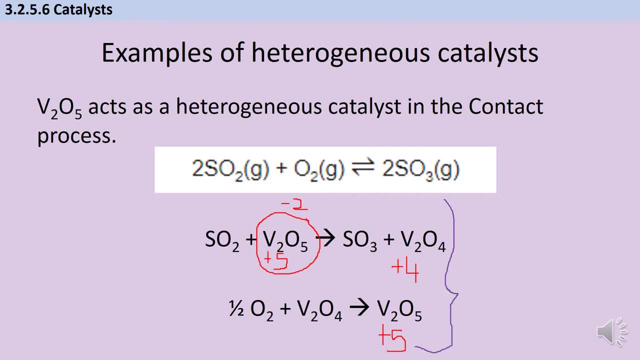 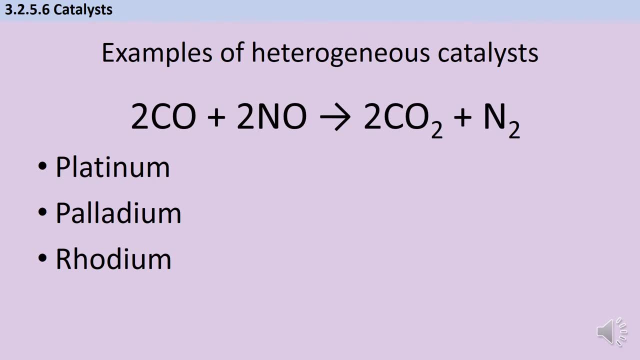 They are in the specification and you just kind of need to write them on a flashcard and memorize them. Here is another example of heterogeneous catalysis, which we've already mentioned, And this is what's going on in the catalytic converter inside your car. 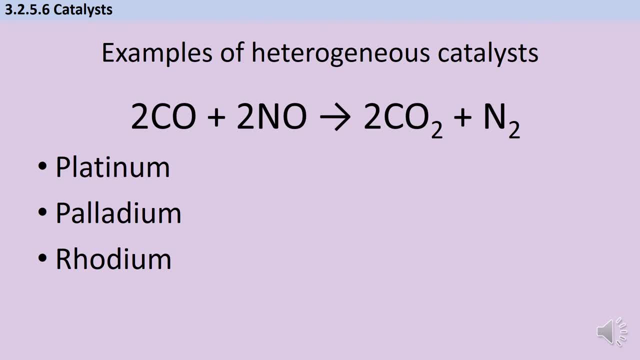 So cars produce carbon monoxide from the incomplete combustion of hydrocarbon fuels and also nitrous oxides Just because it's so hot in the combustion engine that the nitrogen and oxygen in the atmosphere will react together, And neither of those are any good for you at all. 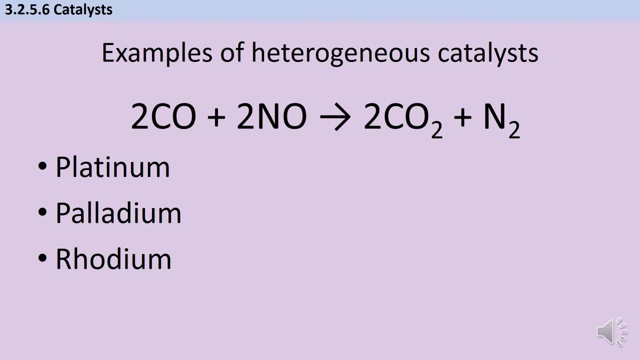 So in the catalytic converter in a car you either have platinum or palladium or rhodium nanoparticles mixed into a paste and then spread over that sort of ceramic support that we saw a little bit earlier And the carbon monoxide is going to be oxidized to make carbon dioxide. 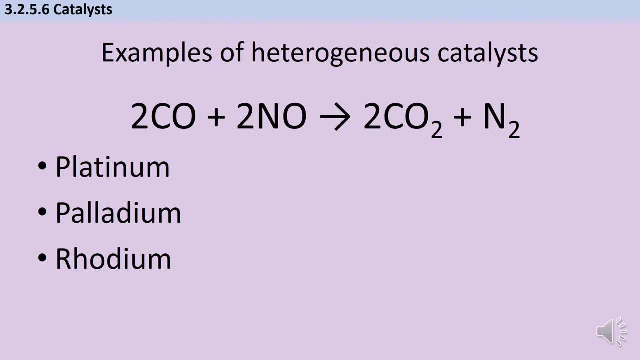 And the nitrous oxides. the nitrogen in them is reduced to produce nitrogen gas. You might be aware that fuel companies now have to remove lead and sulphur from their fuels before they're sold, And the reason for that is because those two elements can poison the catalyst in the catalytic converter. 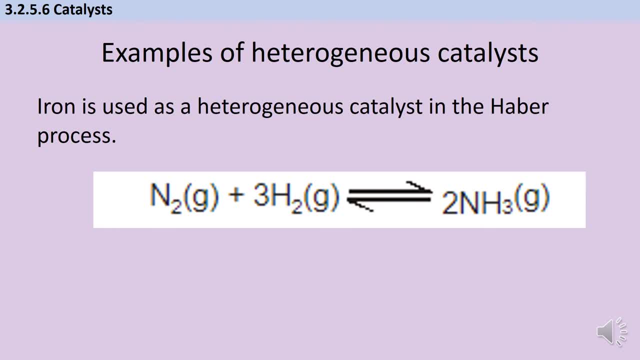 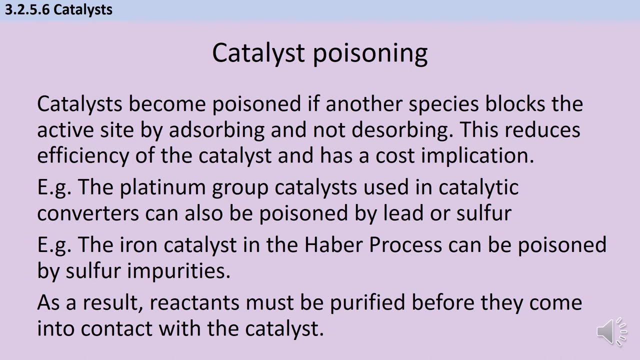 If you took GCC chemistry- what we call triple science rather than combined science- then you would have learned about the Haber process, where ammonia is made from the reaction of nitrogen and hydrogen, And iron is used as a catalyst in this process. For a lot of these examples of heterogeneous catalysis, there is the potential for the catalyst to become poisoned. 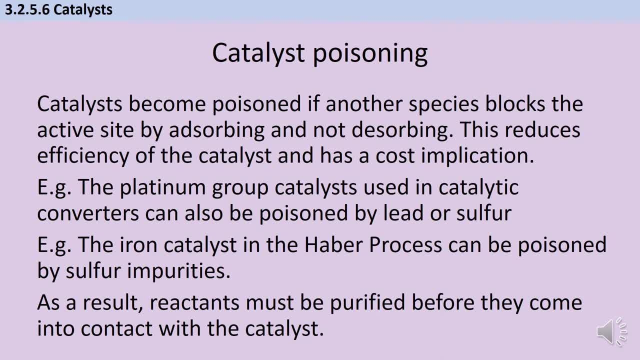 at which point it's going to be far less efficient And that's obviously going to have a cost implication for industry. The best analogy I can think of for this is if you think about what happens if you breathe in carbon monoxide. Your red blood cells contain a molecule called haemoglobin. 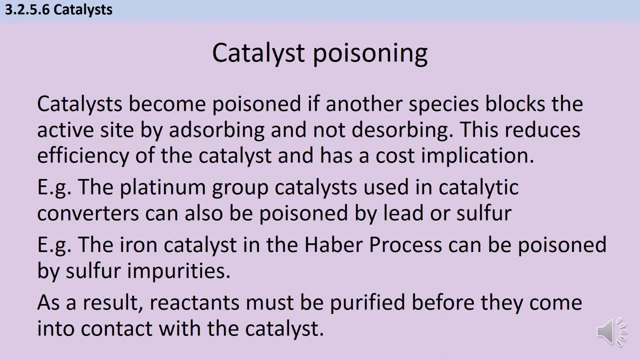 And haemoglobin, under normal circumstances, bonds with oxygen to make oxyhaemoglobin, which is transported with your red blood cells around your body to give your cells oxygen. Unfortunately, haemoglobin can also bond to carbon monoxide And when it does so, it's actually a stronger bond and the carbon monoxide never dissolves. 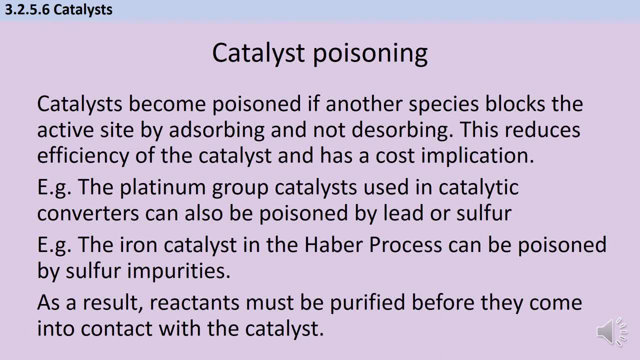 It never lets go, And so the haemoglobin is unable to bond. It's unable to bond to any oxygen And it kind of goes out of action And the red blood cell that has that haemoglobin is just kind of useless. 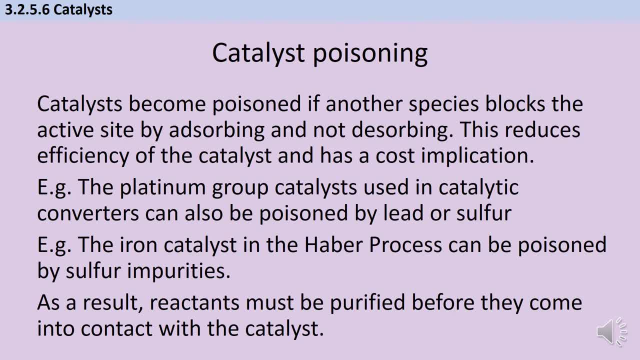 It can't carry any more oxygen. And this is exactly what happens when a catalyst gets poisoned. Another species comes along which adsorbs to the active site of that catalyst, And then it just doesn't desorb, And so that active site is blocked. 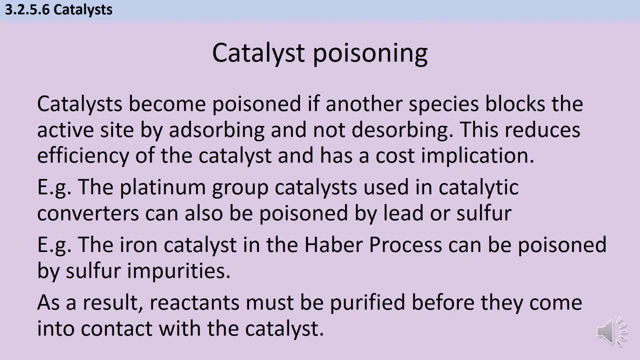 And the catalyst as a whole is going to be less efficient because that particular catalyst is unable to work anymore And it just kind of makes the whole thing a bit useless really. So some examples of this: We talked about how catalytic converters in cars have platinum group metals like platinum, palladium, rhodium in them 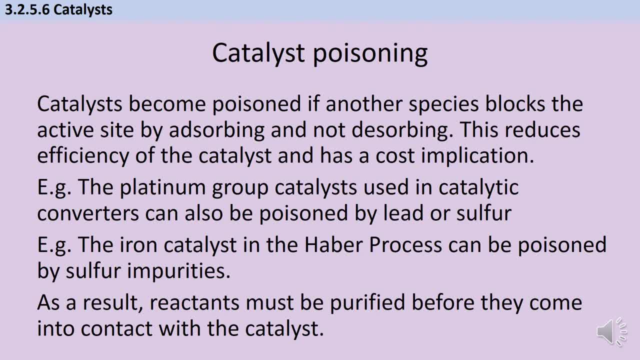 And those can be poisoned by lead or by sulphur, And also the ion catalyst in the Haber process can also be poisoned by sulphur. Now, once a catalyst has been poisoned, there's not really a lot you can do about it. 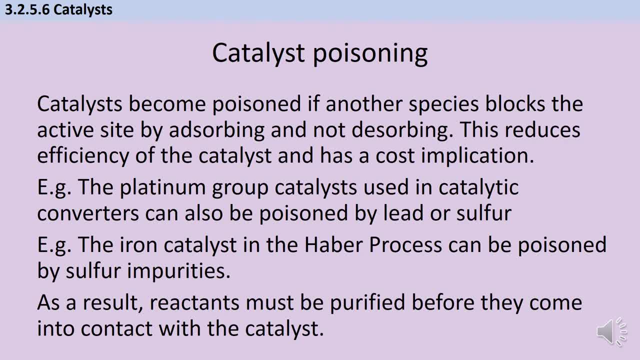 You can't sort of unpoison it. So it's really, really important, if you're working with a catalyst that could easily be poisoned, that you do something to make sure that the reactants have been purified, so that the reactants aren't going to. 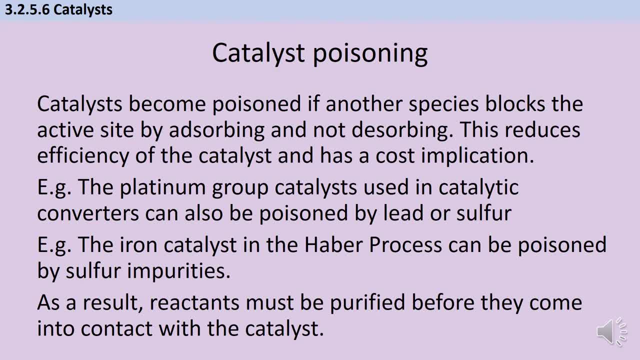 you know, poison the catalyst in the first place, And so if you think about if you are filling up fuel, then you know that you can buy petrol or diesel that is described as being unleaded. Now, 20,, 30 years ago, you could also buy leaded petrol. 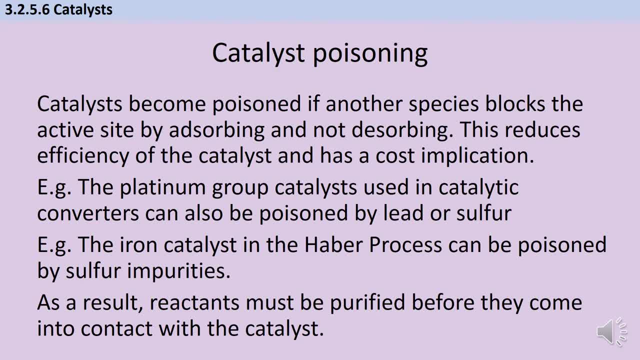 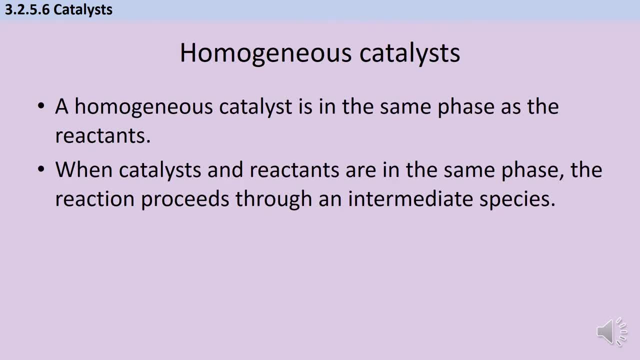 And so the reason that we now have unleaded petrol is because the fuel companies are actively removing that lead so that it can't poison those catalysts. As we said about 10 minutes ago, the homogenous catalyst is in the same phase as the reactants. 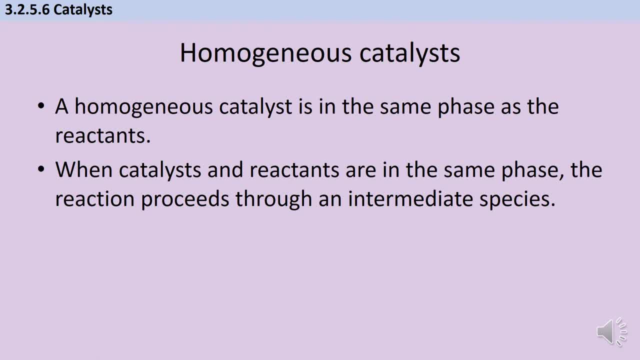 So we're usually going to be talking about a catalyst which is itself dissolved. It's in the aqueous phase, And so are the reactants it's working with, And when the catalysts and the reactants are in the same phase, then the reaction is going to need to proceed through an intermediate species. 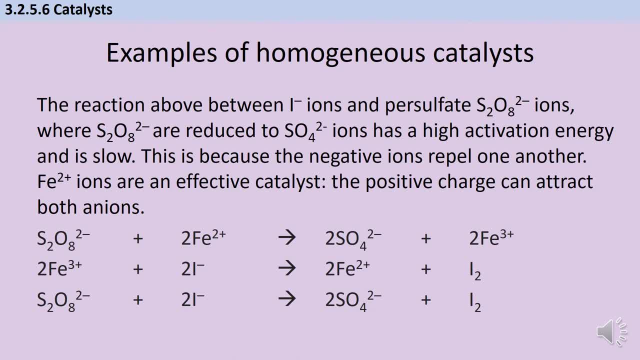 Here's a classic example of homogenous catalysis: Iodide ions are able to reduce persulfate ions down to make sulfate ions and, in doing so, themselves are oxidised to make iodine Following. so far, Unfortunately, both the iodide ions and the persulfate ions. 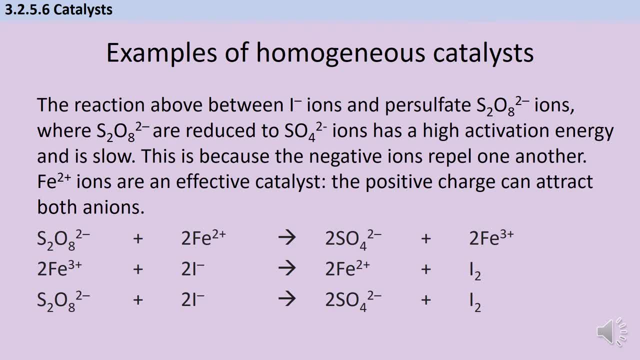 are anions, They're both negative And, as we know, two negative things are always going to repel each other. So it takes a lot of energy in order for those anions to be able to interact And therefore the activation energy for this reaction is very high and therefore the reaction is very slow. 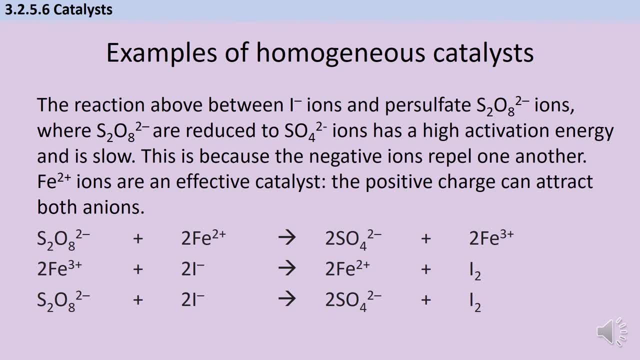 But the only thing that's stopping it from happening is the fact that those negative ions are repelling each other. So if you have a positive ion, if you have a cation, then they would both be attracted to that cation, And this is where our transition metals come in. 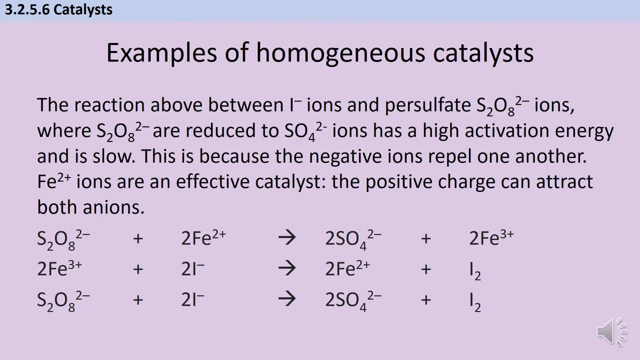 So ion ions make really quite a good catalyst for this reaction. So if we break this down into some half equations we can have: our persulfate ion is going to be reduced by iron two plus. So the iron two plus is acting as a reducing agent and is itself going to be oxidised to make iron three plus. 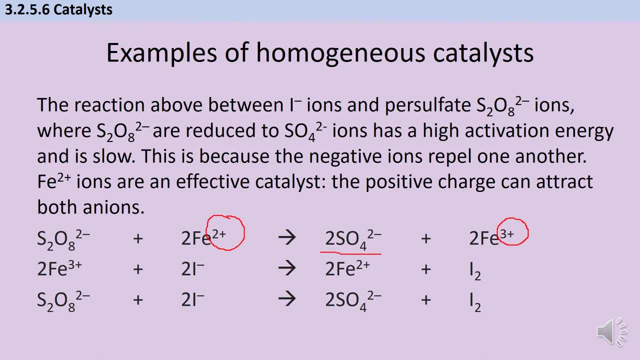 And the persulfate ion is reduced to make sulfate ions And then at the same time, those iron three plus ions are going to be a useful catalyst. They're also going to attract anions and they're going to attract these iodide ions. 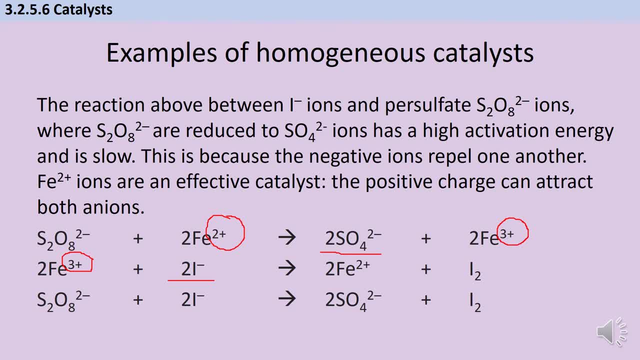 And in doing so, the iron three plus is going to act as an oxidising agent and is going to oxidise the iodide ions so that they end up being turned into iodine. So my, my iron two plus is acting as a reducing agent. 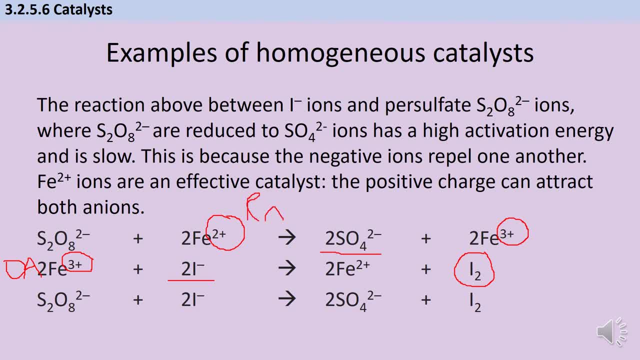 And my iron three plus is acting as an oxidising agent And if we put those together then we can have an overall ionic equation, which is my persulfate ions being reduced to make sulfate ions and my iodide ions being oxidised to make iodine. 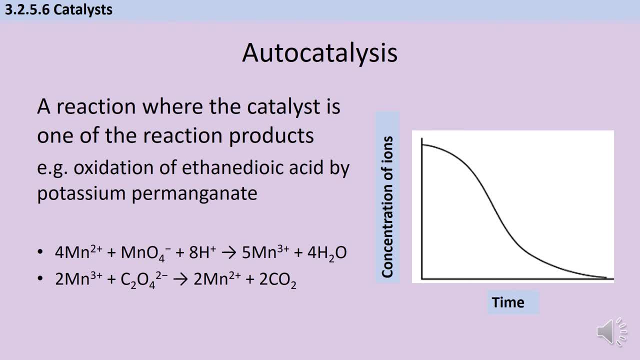 Some chemical reactions are autocatalytic. Auto always means doing something to yourself. So, for instance, you write a biography about somebody else's life, but an autobiography you don't. An autobiography you write about your own life. So an autocatalytic reaction is one that's literally catalysing itself. 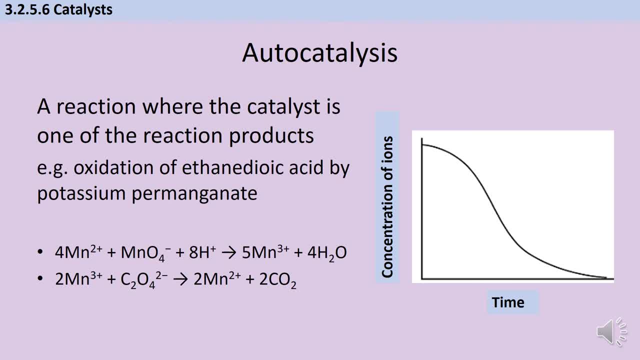 And the reason it's catalysing itself is that the catalyst is one of the products being made, And what that means is that as the reaction proceeds and more and more product is made, then it's going to go faster and faster. So if you look at a graph of the concentration of the reactant,